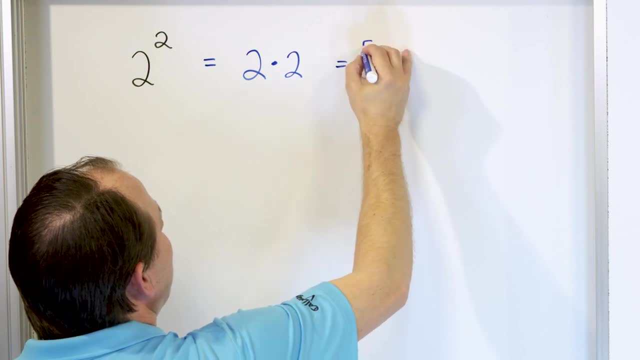 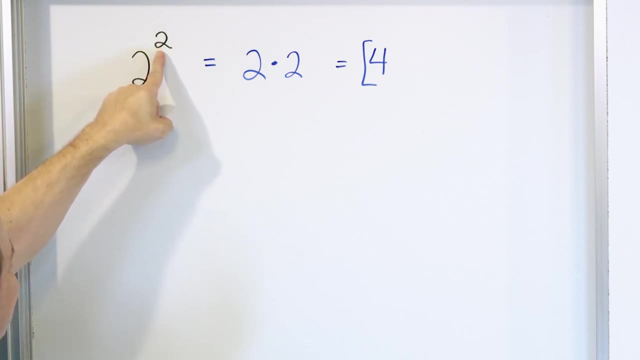 And then of course, you know what two times two is and you just write down that the answer is four and that's the answer. So if you go into a calculator or a computer and you put two and raise it to an exponent power of two and calculate the answer, 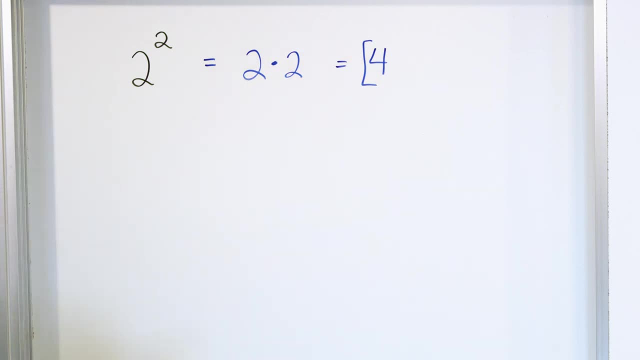 it's going to be the same thing as two times two, which is going to be the same thing as four. So the idea is: exponents allow us to write down multiplications when it's times itself, lots of times, or very, very quickly and easily, And also we use it very, very, very often in real 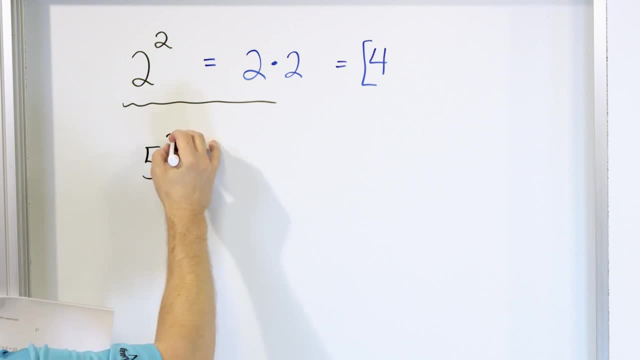 life problems. Let's say we have the problem five raised to the power of two. Now, the power of two is actually really important because it's going to be the same thing as two times two and it's really really common. It's so common actually that we call it as a special word. So 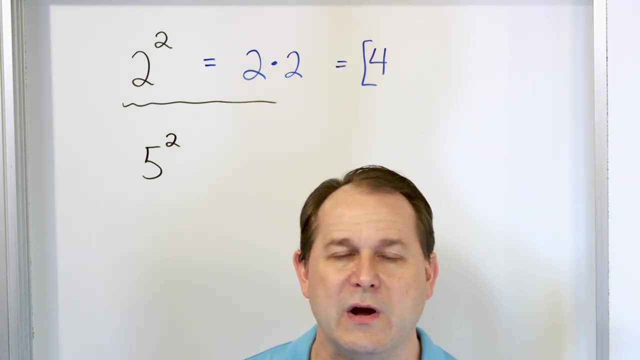 five to the power of two, or five raised to the exponent of two, we call it squared. So if somebody tells you, hey, what's two squared, What's three squared, What's four squared, All it means it's raised to the power of the exponent of two. And again, there's so many examples of that. When I 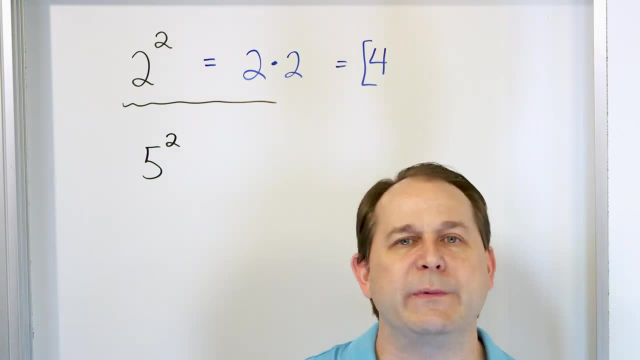 throw a baseball and it makes a curved arc in the sky. when we write down the math that describes the curved path, we have exponents that are raised to the power of two, And so, if you're going to write down the math that describes the curved path, you're going to have exponents that 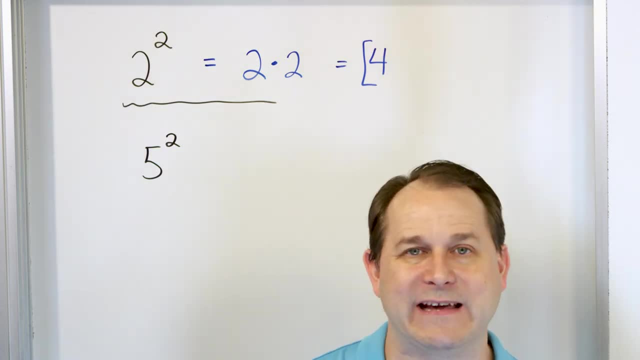 are raised to the power of two, running around all of our math that we use to calculate things like that in real life. So here five to the power of two means what It means. we take the base five and we multiply it by itself so that it's done here two times. We have two fives here. 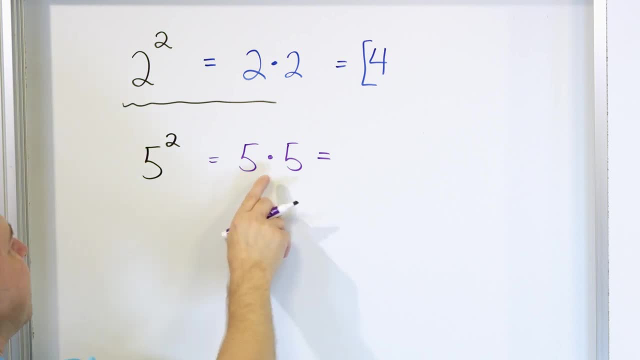 because it's raised to the power of two. Five times five, as you know, is 25.. So we now know that five squared, or five to the power of two, is 25, just like two squared, Also the same thing. 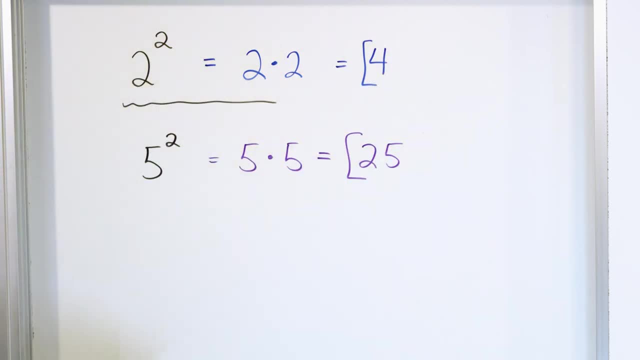 is two to the power of five, So we have two squared and we multiply it by itself so that it's four. sorry, two to the power of two is equal to four. All right, these are really simple problems, really fast problems. Once we get the hang of it, it's going to go really fast. Problem number three: 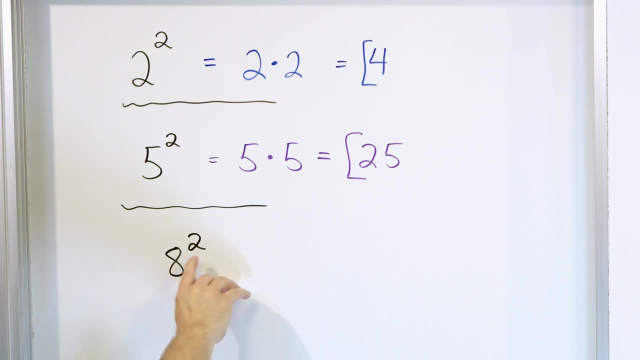 what if I give you eight raised to the power of two Again? so far all of the exponents have been two. So here, what do we do? It just means you take the eight, which is the base, and you multiply. 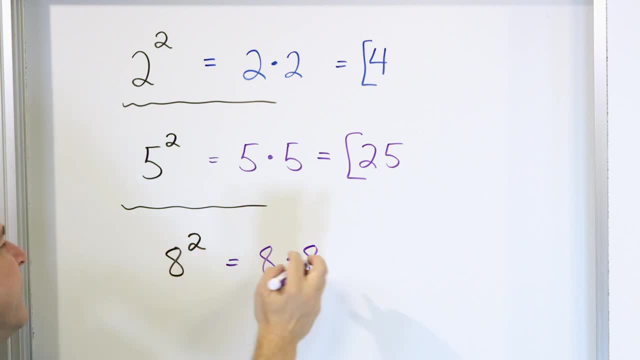 it by itself. and how many eights do you have Two of them, And so you multiply eight times eight and you get 64. And so we've learned that eight squared, or eight to the power of two, is equal to the number 64. So you see the pattern You're just. 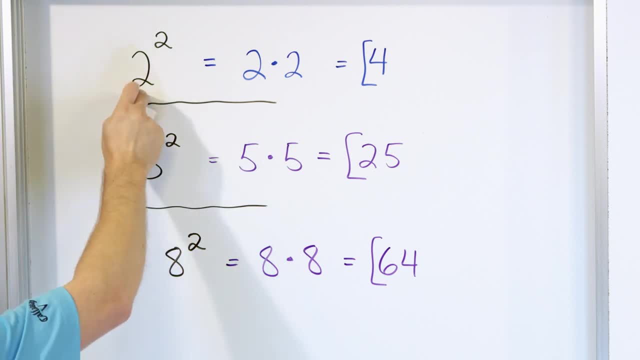 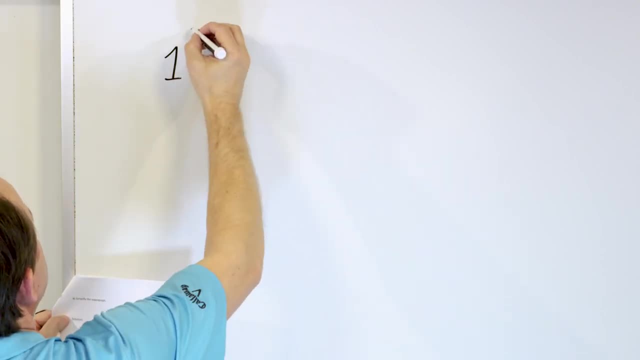 multiplying it by itself, It's eight times eight, five times five, two times two, and the exponent tells you how many times to do that. Now, here we have a little bit of a different animal. What if I give you the number one into the power of three? What do you think is going to happen here? 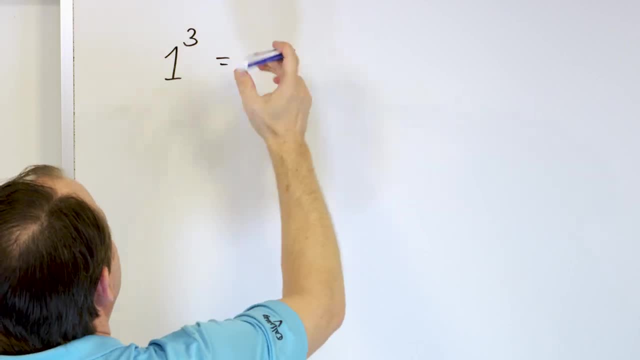 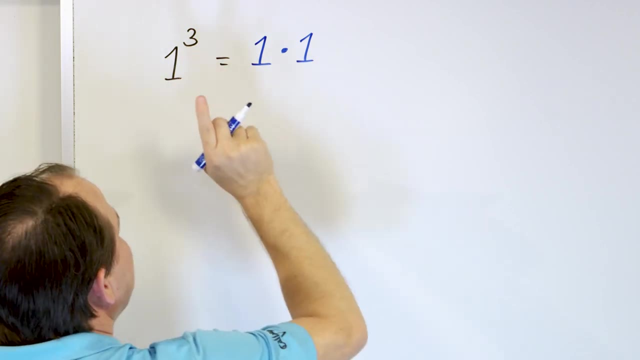 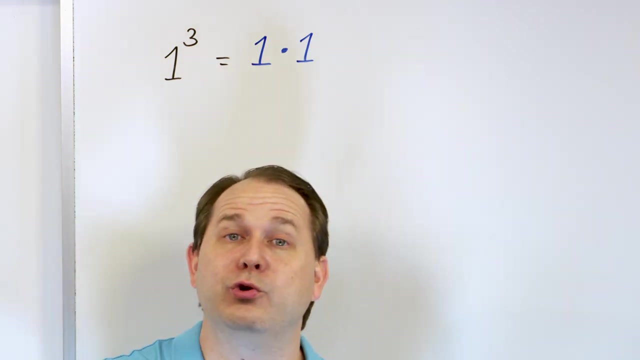 Well, basically what we do is we still multiply by itself. but how many times do we do it? Here's a one, Here's another one. That would be one squared, but we don't have that. We have one cubed. Cubed is another way of saying power of three, So squared is power of two Cubed. 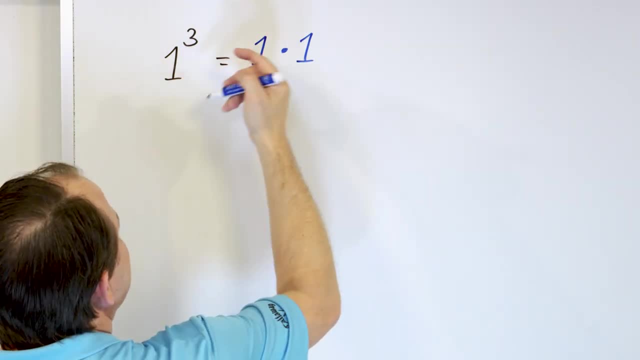 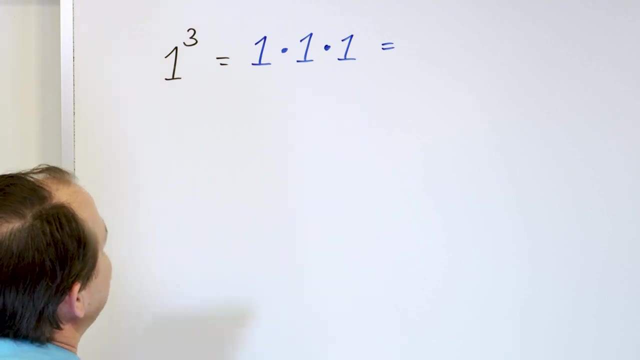 is power of three. Those are just words that we have here Since it's cubed. we actually have to multiply another time because there has to be three ones here since it's cubed. Now we follow order of operations, We have multiplications, We go left to right. So one times one is one, We still 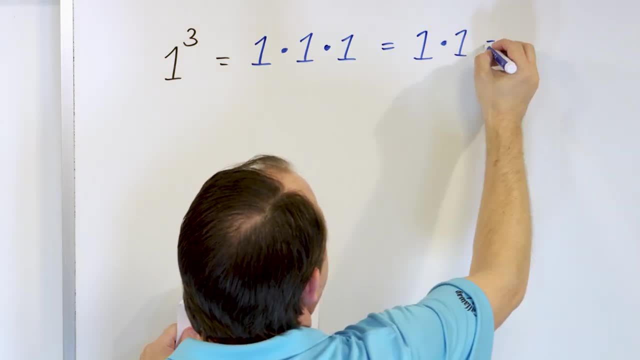 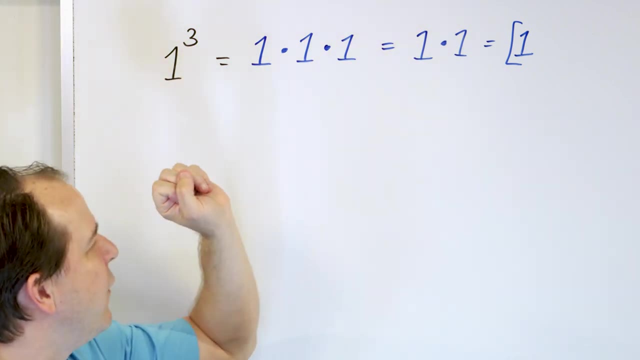 have that one left over. We just calculated this one and now we have one times one, which again is one. So here's a bonus question. One to the power of three is what One? What do you think? one to the power of four is? Well, you just multiply by one again, You'll get a one. One to the power of five: 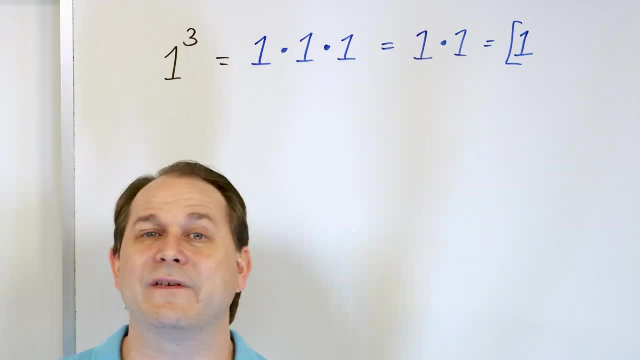 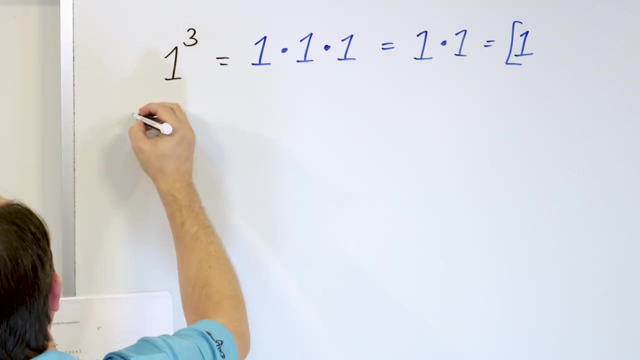 still one. One to the power of seven, still one. One to the power of a thousand? still one, because multiplying by one just doesn't really change much. All right, next problem, Let's take a look at something a little different. What about two to the power of three? Well we're. 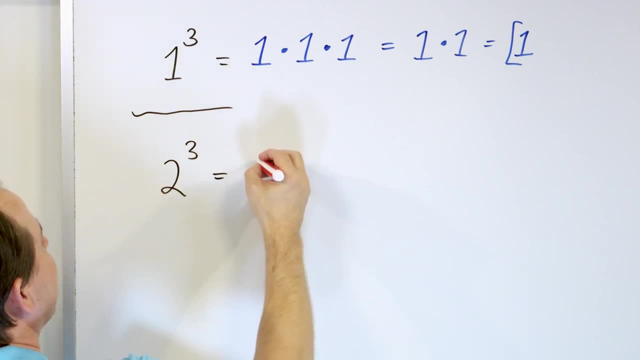 multiplying again by itself, Times itself. Here's a two. Multiply by a two That would be two squared, but we have two cubes, so we have to have another two. there Again, we follow order of operations. We multiply. left to. 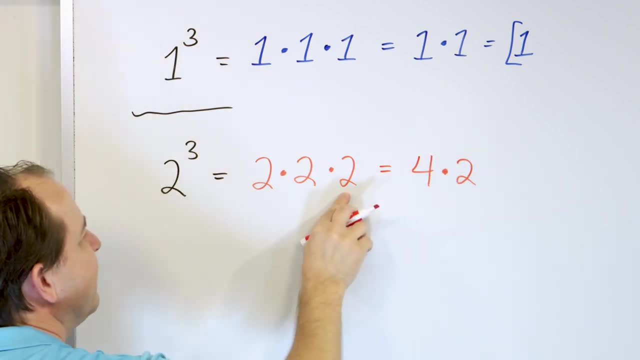 right. Two times two is four. We still have this times two here that we have to do, So this was four times two. Four times two is eight. So two to the power of three or two cubed is eight One. 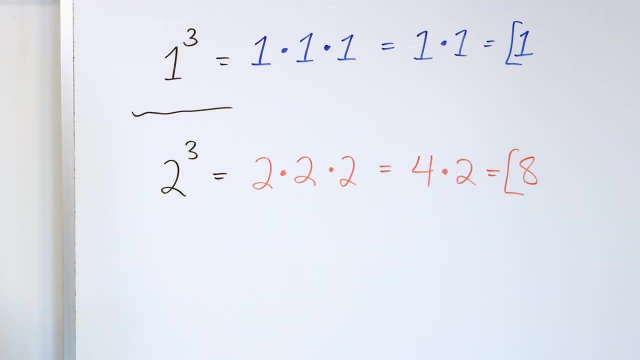 to the power of three or one cubed is one. All right, Let's switch back to square. We have two squares. What do you think seven squared is? or seven to the power of two? Well, again, we always. 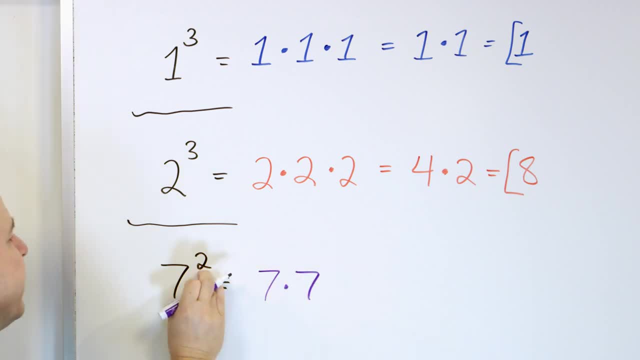 multiply by itself. So it's seven times seven. There's only two of them here, because it's squared. Seven times seven is 49. So the answer of seven squared is 49. So you see the idea of exponents. it really gives a lot of students trouble, but the actual concept is dead simple. 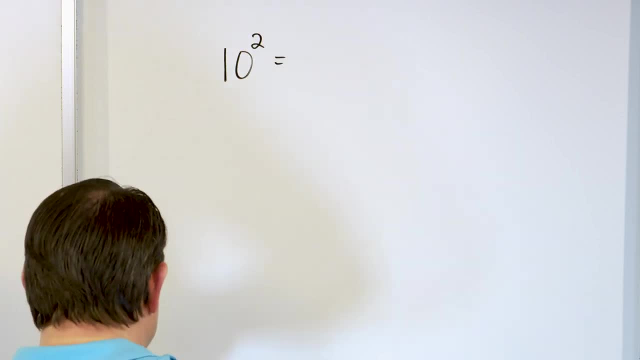 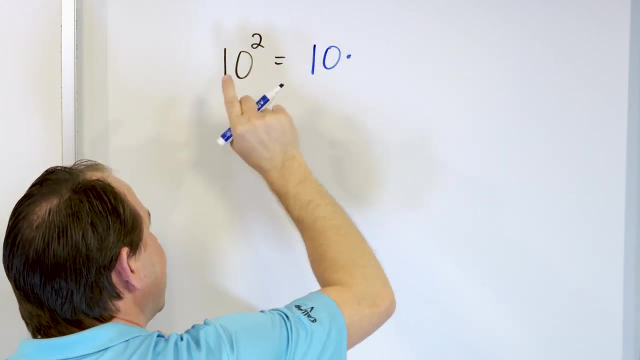 What about 10 to the power of two? I mean, it follows the exact same formula, but it's not the exact same pattern. every time You're multiplying times itself 10 times, not times two, not times two, 10 times 10.. You're multiplying by itself and you're doing it two times 10 times 10. 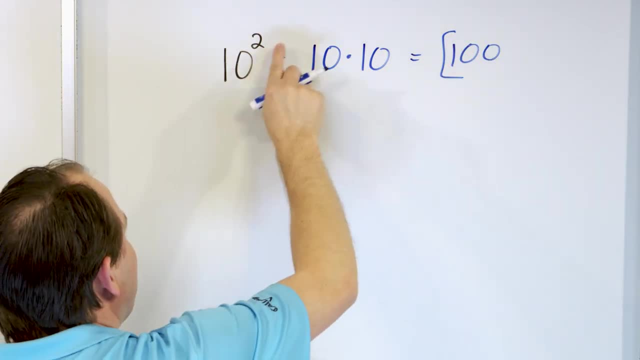 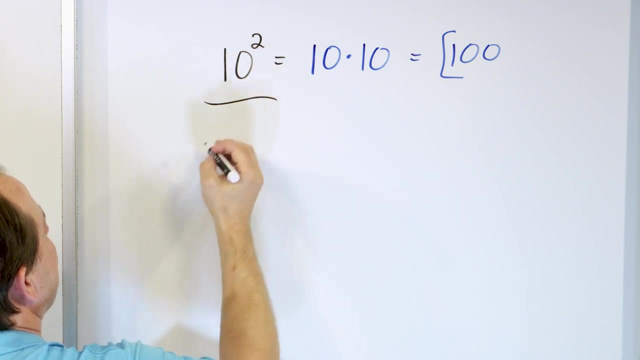 is what? 100.. And so we've learned that 10 squared is equal to 100, or 10 to the power of two is equal to 100.. All right, Let's choose something a little bit larger. What about three to the power of three? What do we do for that one? Again, we're always multiplying by. 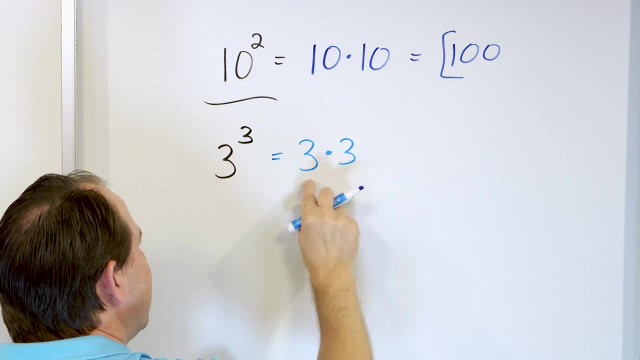 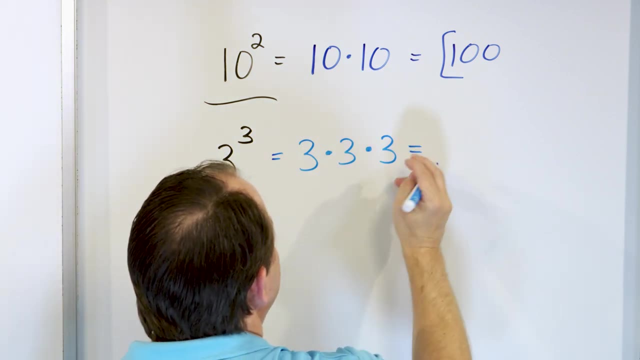 itself. So we have three to the power of three. We're multiplying by itself. So we have three times three. That would be three squared, but we have one more up here. We have to go times three again. There's three of them here. So three times three times three. Let's do. order of operations. 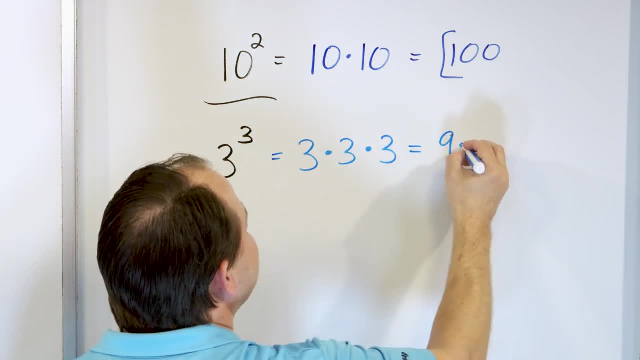 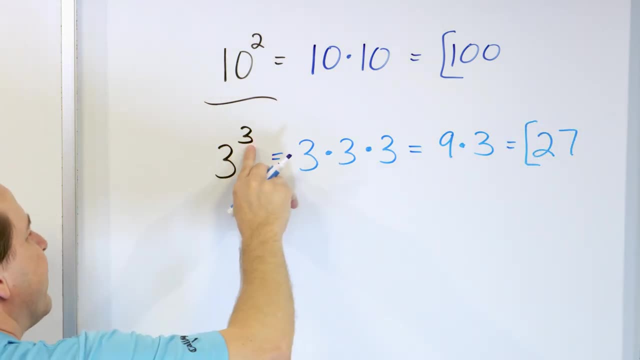 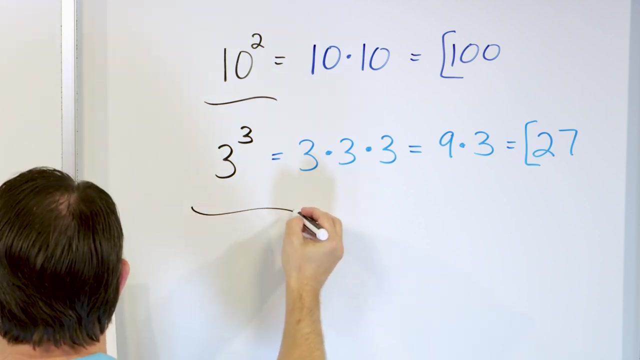 We have to go left to right. Three times three is nine, but we still have this times three there. What is nine times three? It is 27.. So we've learned that three to the power of three, also called three cubed, is equal to 27.. All right, I only have a couple more problems. What about? 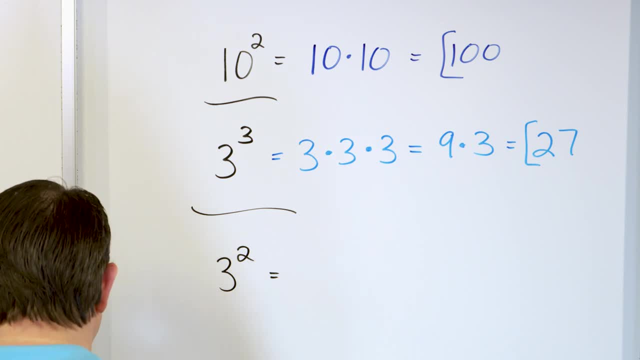 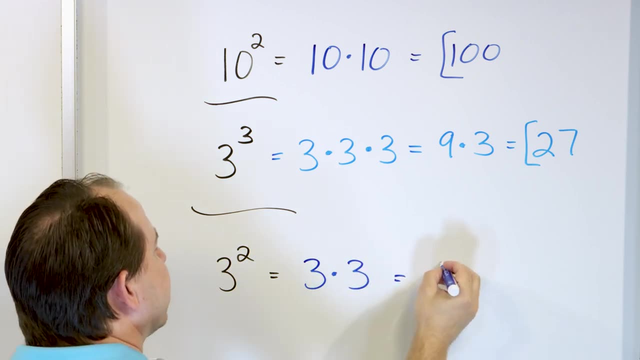 three to the power. Well, it's very similar to what we just did above. Here we only have a square, So it's three times three. There's two of them here, And three times three is nine. So we've learned that three squared. 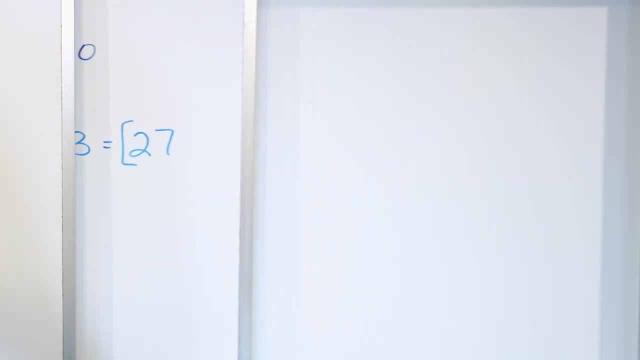 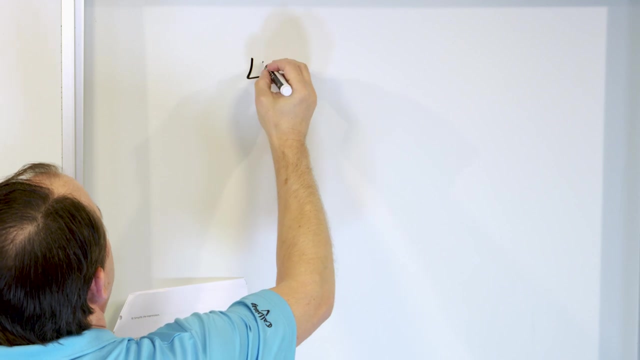 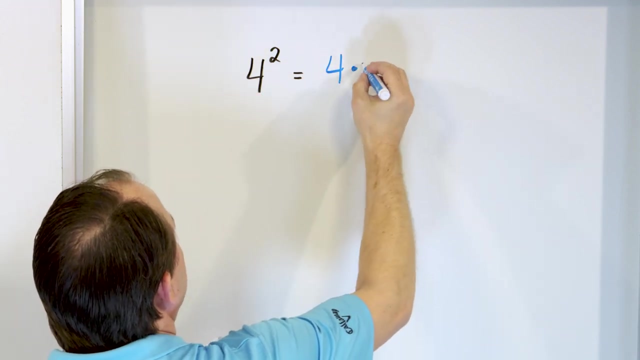 is in fact nine. All right, I think we only have one more problem here. What about four to the power of two or four squared? What is that? Well, it's going to be again multiplied by itself Four.